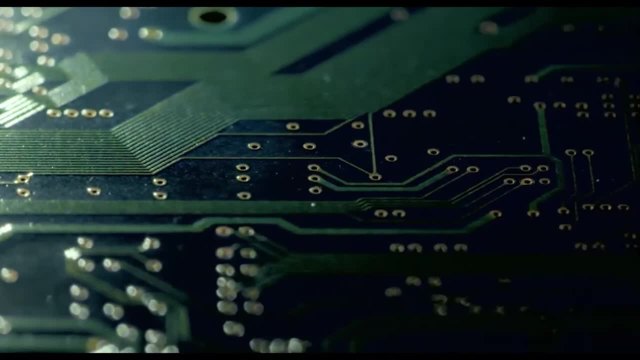 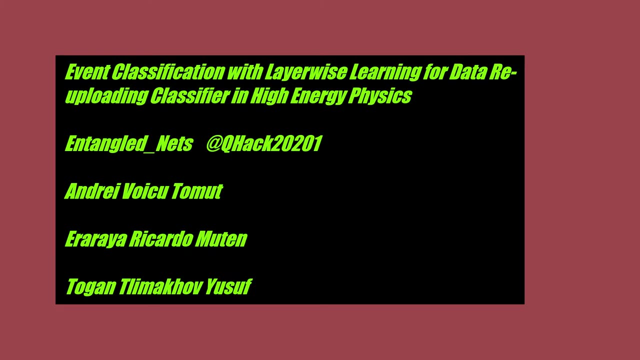 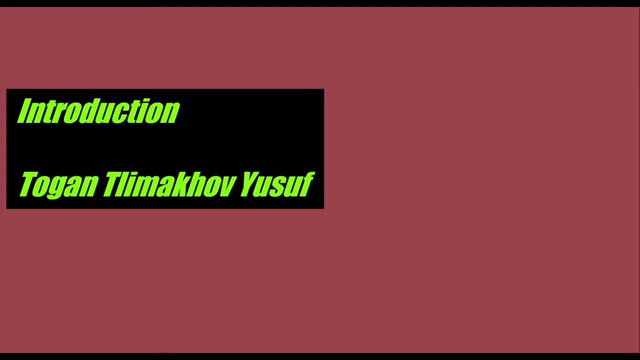 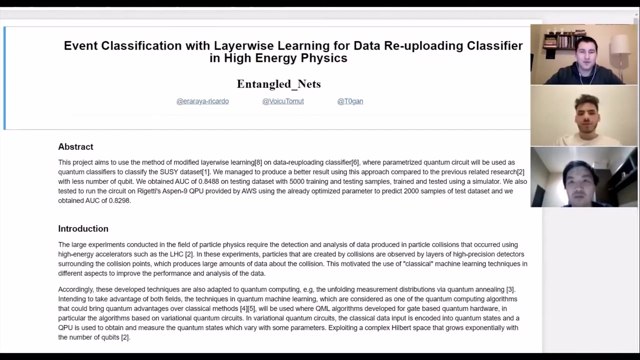 All right? Hello everyone, My name is Togan and I am a member of the Integra NETS team. Today, we are going to present our project idea within the scope of QHACK 2021, organized by Xanadu. 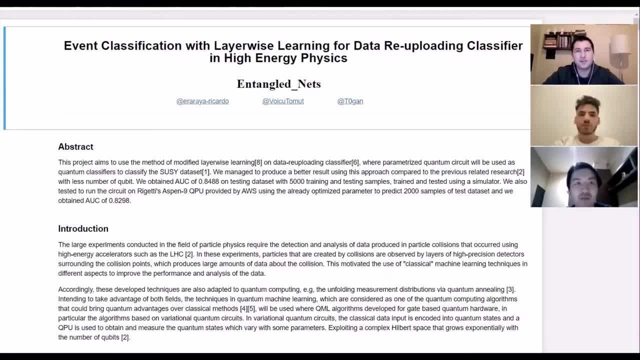 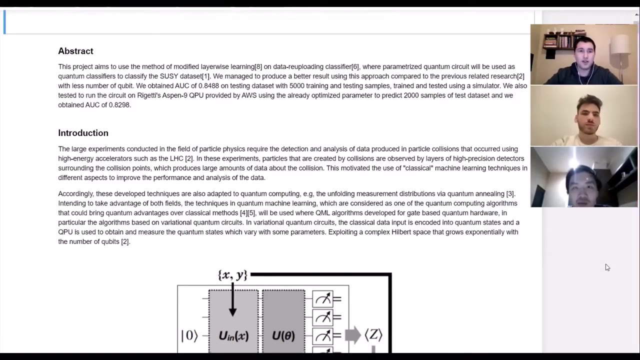 Our project is titled Event Classification with Liarized Learning for Data Reuploading Classifier in High Energy Physics. Initially we had this idea. We wanted to solve a real-life problem. We checked a data set given at CERN. So, as we know, the large experiments concluded in the field of particle physics produce a large amount of data after the collisions, such as the experiments done in the LHC. 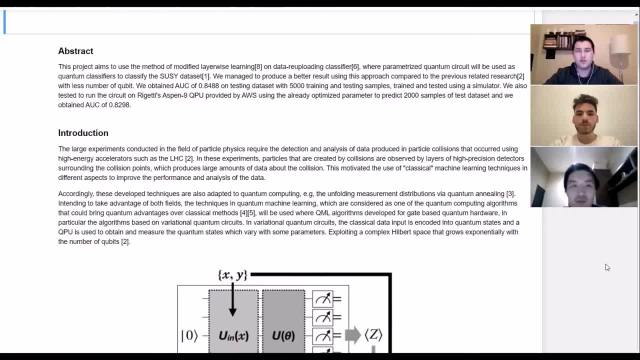 These huge amounts of data have motivated the usage of data, So we decided to use classical machine learning techniques in different aspects to improve the performance and the analysis of these data. Now, accordingly, the methods of quantum computing have been started using in the last decades or so to help provide more improved analysis of these data. 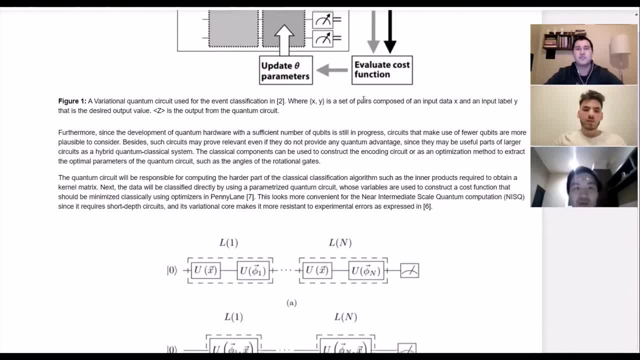 Therefore, since the development of quantum hardware with sufficient number of qubits is still in progress, we think that we can use a method that will use the computational power of single qubits. Now, therefore, we use the method of data reuploading. 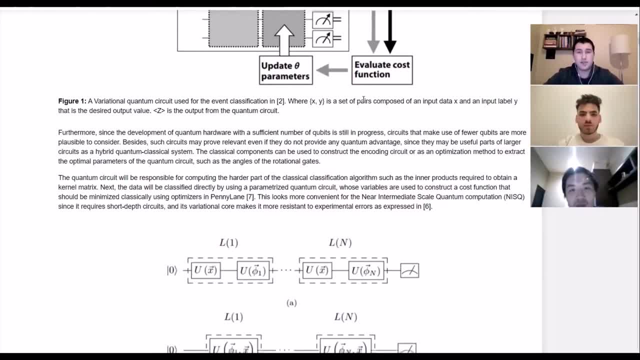 And the way it works, as we all know, a quantum state is represent is characterized as a single state. So the way it works, as we all know, a quantum state is represented in a is characterized as a single state. 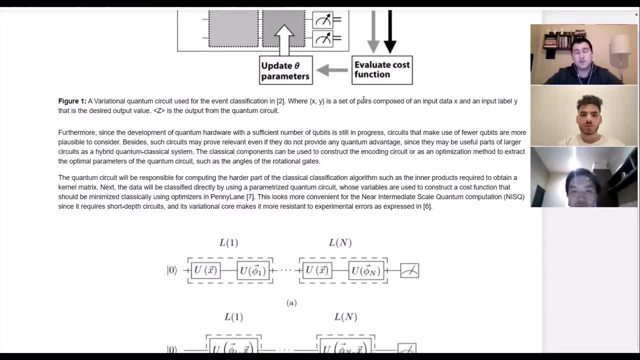 two-dimensional state vector and can be visualized as one point in the Bloch sphere is. in order to load the data onto a single qubit, we use unitary operations. now let's say we start with the state zero and we want to modify the state of the qubit on the Bloch. 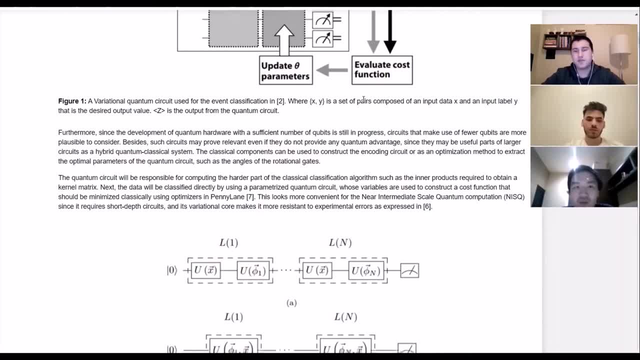 sphere we apply a neutral operation with the specific parameters that will. these parameters will be, as a parameterized matrix, multiplication, representing the rotation of the state vector in the Bloch sphere. so, for example, if we start with the state zero and applied specific unitary operation with the different parameters, we will end up at a different point in the Bloch sphere. 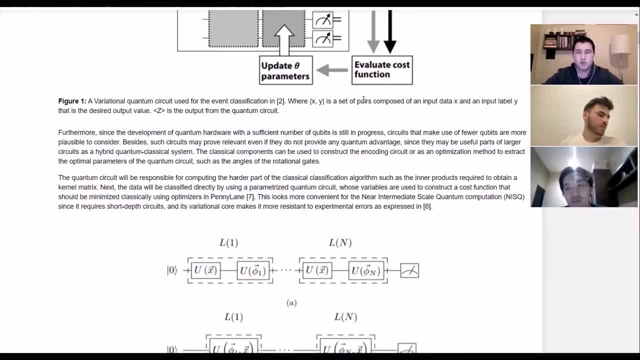 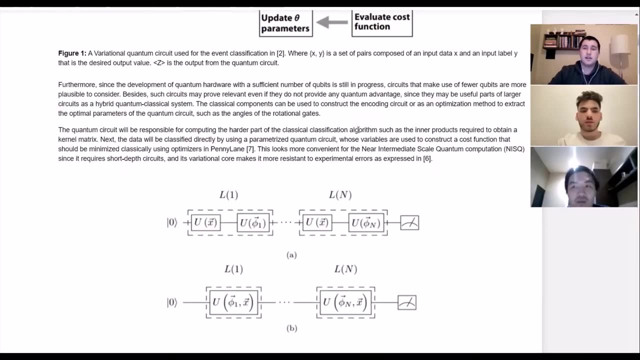 and applying more than one unitary operation will modify the state of the qubit this way. so we want- of course this cannot be only used for one single qubit, but then for multiple qubits, and this is what we try to use to- to use this variation quantum circuit as a 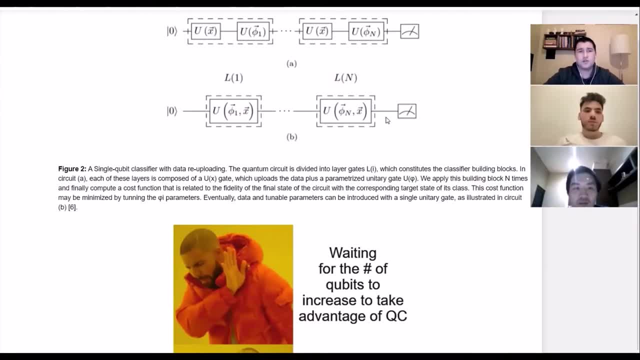 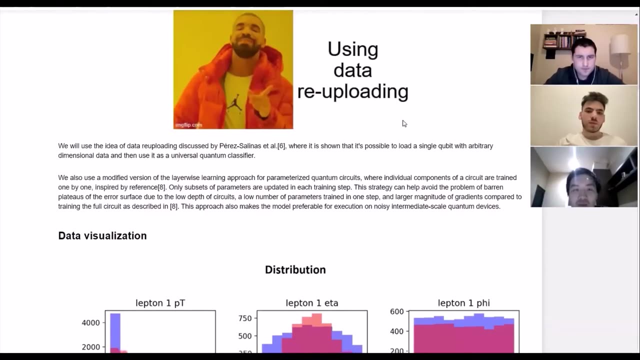 classifier as a universal classifier, universal quantum classifier, to classify the data we we obtained from the data set called SUSY. all right, besides all the re-uploading technique, we have also modified version of the used modified version of layerwise learning approach for parameterized quantum circuits, where individual components of the circuits are trained one by one. 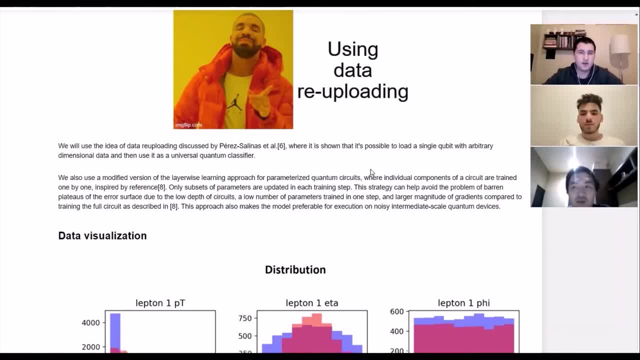 inspired by the reference article number eight, where only subset of parameters are trained one by one. inspired by the reference article number eight, where only subset of parameters are trained one by one and the training steps are uploaded in each training step. this transition can help us avoid the problem of barren, flat use of error surface due to the low depth of the circuits. 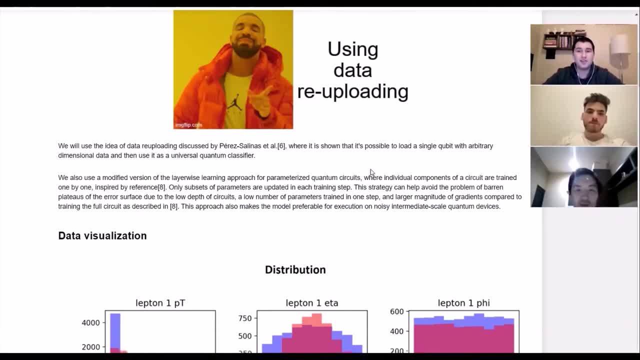 a lower number of parameters trained in one step and a larger magnitude of gradients compared to the training of the first circuit, as described in article 18 as well. of course, this approach also make the model preferable for execution on a noisy intermediate scale quantum devices similar to the reuploading data technique. 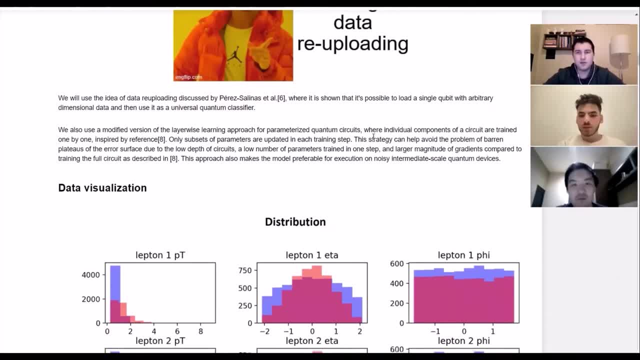 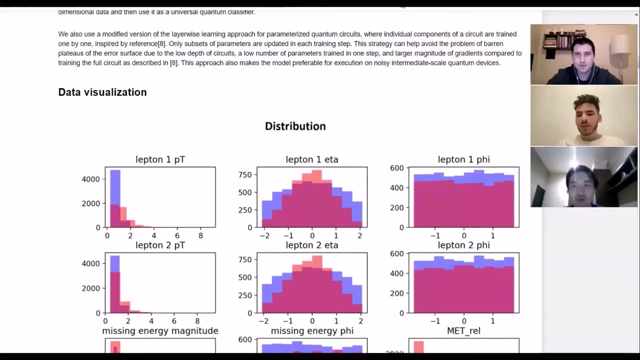 Okay, now I will leave. I will pass it to Andrei to explain us the circuit and the data visualization in depth. Hi, I am Andrei and I will present the data that we have, more precisely the SUSY dataset. that is free and available. 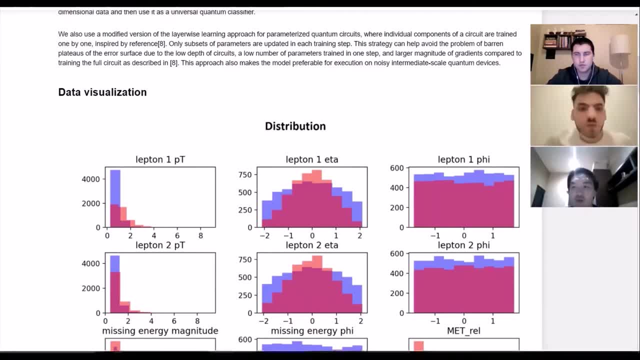 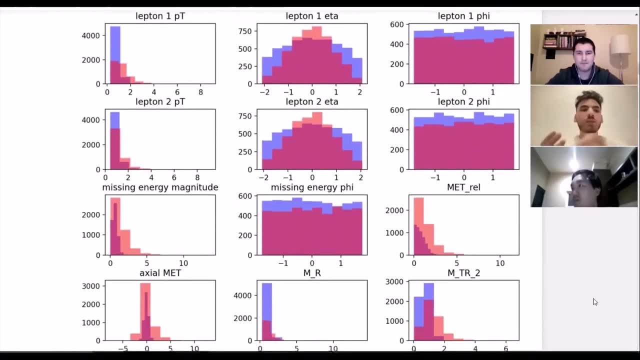 So what we want to do? we want to find if our collision resides in a desired particle or not. For this we can measure direct the particle, because he has a short time span, but we can measure the decay products And how we measure things. so we put some sensor and we identify some parameters. 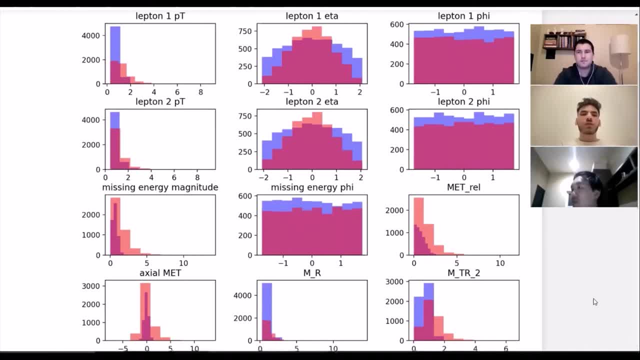 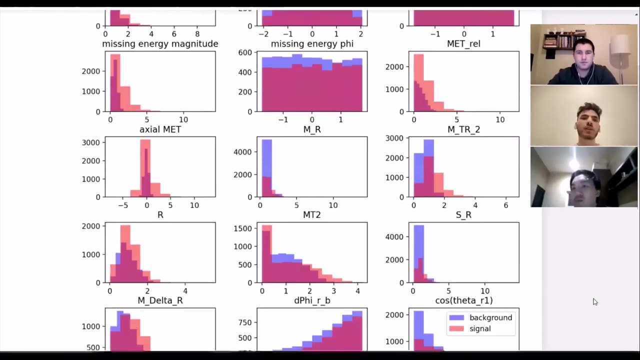 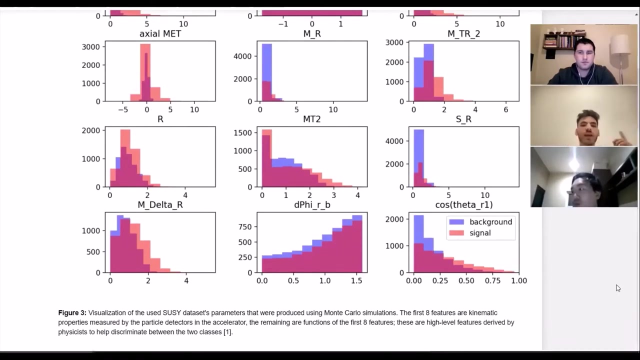 For example, the momentum of the point in some spot, And we can identify that, We can identify the direction. But in SUSY dataset these data are not taken from a real device, are simulated using Monte Carlo, And here I have some graphs, some histograms with the distribution of the background signal and the signal that comes from a successful collision. 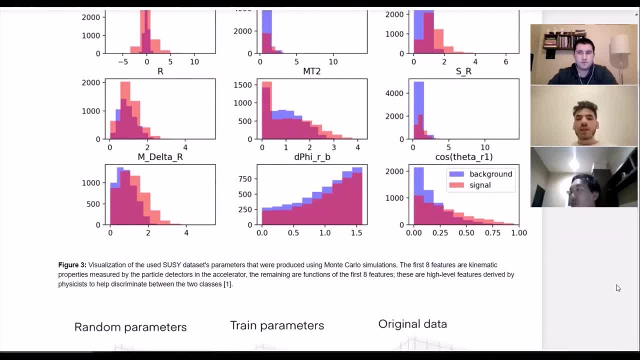 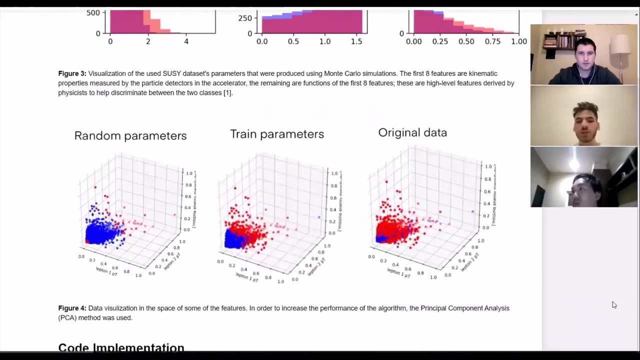 Okay, So from these 80 parameters, just eight are first parameter and the second 10 are generated from the first eight. The most important parameters, as we can read in the paper that inspire us, are the momentum of the lepton one and lepton two. 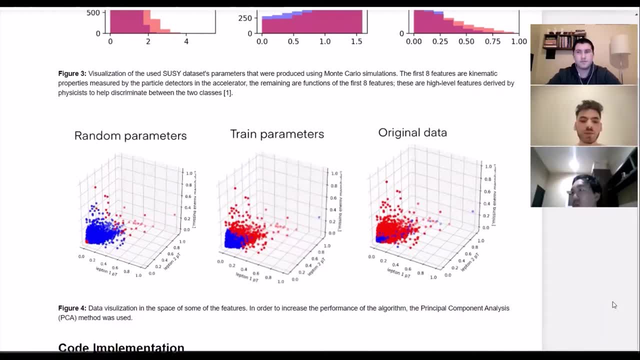 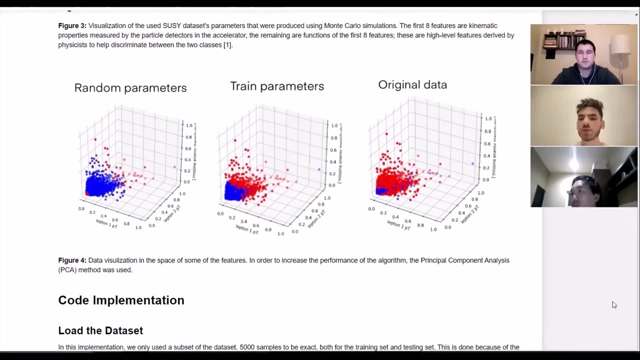 These are the three basic parameters, but we also make tests with more parameters And if we look in these graphs, we have a representation of the data- original data- in the right part of the screen When we have this momentum on the axis and missing energy on the z-axis. 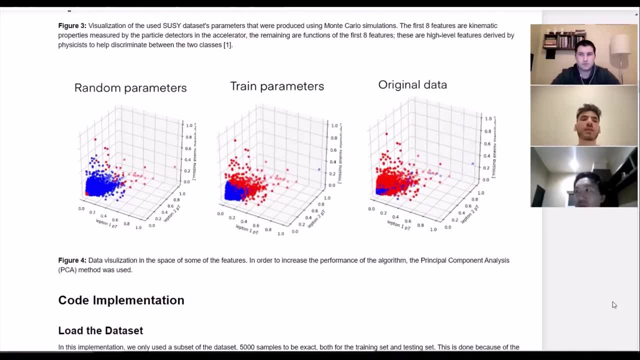 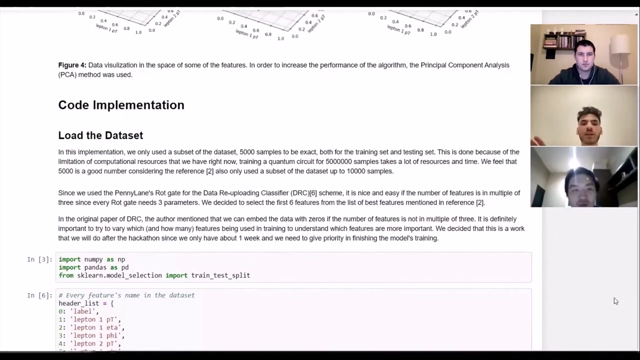 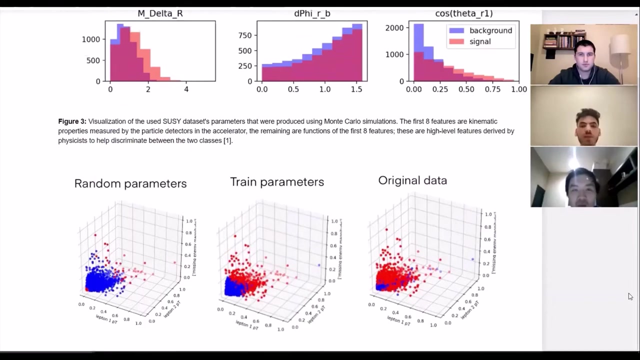 We also try to apply PCA, but we don't get a lot better results using PCA. The other parameters that the first parameter are polar, respective azimuthal angle- And sometimes we use eta instead of polar angle- And measuring the difference in potential From the particles that are registered by our sensor. we can calculate the missing energy that appear from the particles that are generated and we cannot observe them. 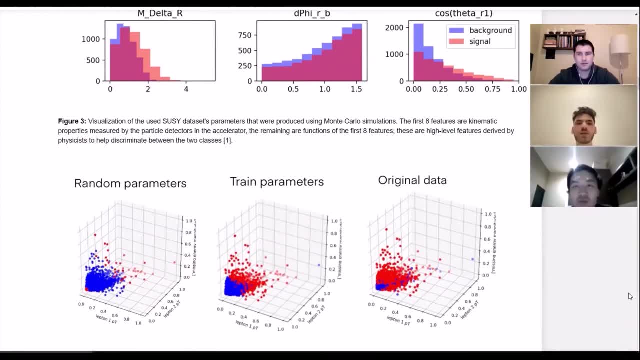 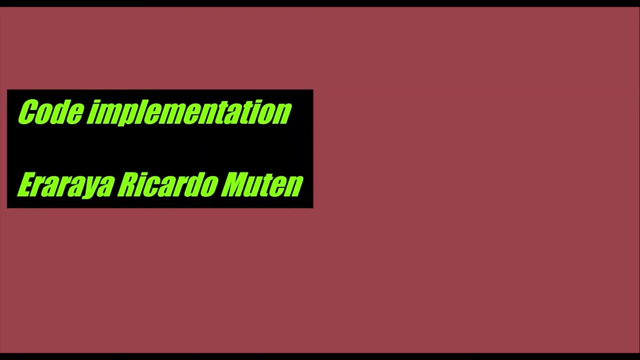 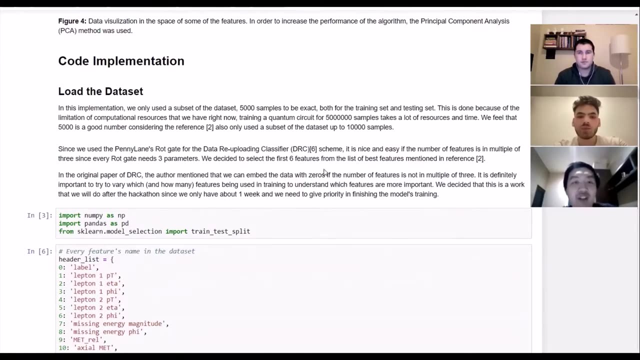 Okay, Now I will let Edu to explain the code. Thank you, Andrey, for the explanation for the data sets. So in our implementations we only use a small number of subsets from the whole data sets. This is because we have little time and small resources. 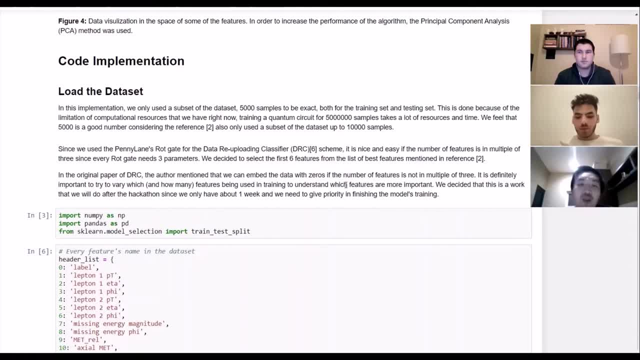 So we choose to use just 5,000 samples For both the training set and testing set And we don't use the whole 5,000,000 of samples because it will take a lot of resources and time And we feel that 5,000 is quite a good number considering the reference paper number 2.. 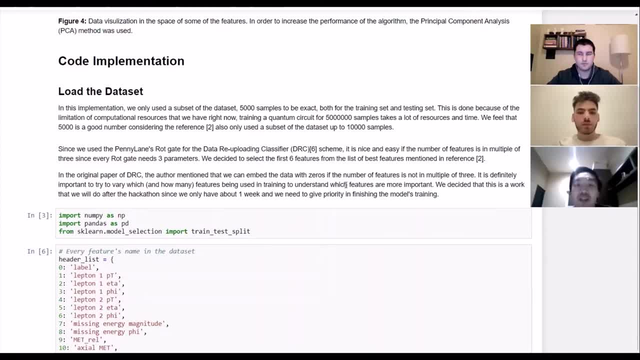 So only use a subset of the data set up to 10,000 samples. Since we use the Penny Lane's route gate or the rotation gate For the DRC, it is nice if we use, if the total number of features we use is the multiple of 3.. 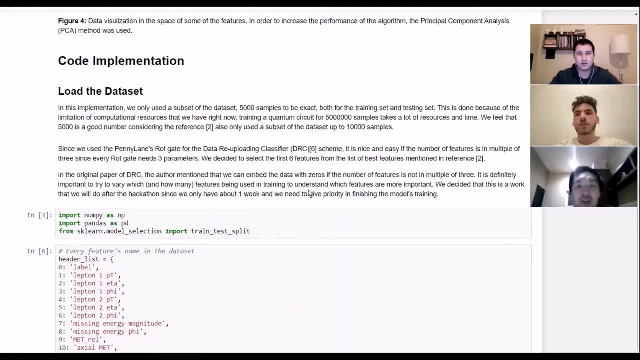 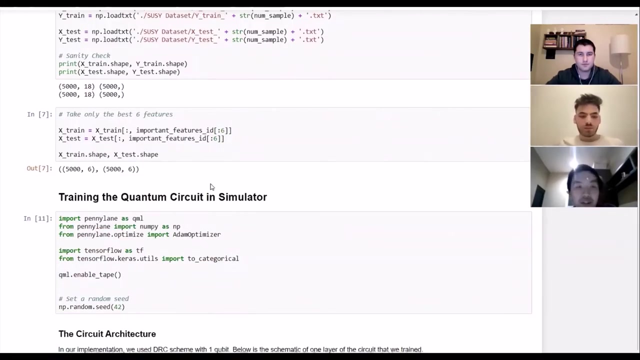 But we realize that in the future works we also need to analyze what features is more important And how the number of features impact the data set And how the number of features impact the training accuracy. Okay, And in our implementation we decide to use the top 6 best features. that is proposed by the reference paper number 2.. 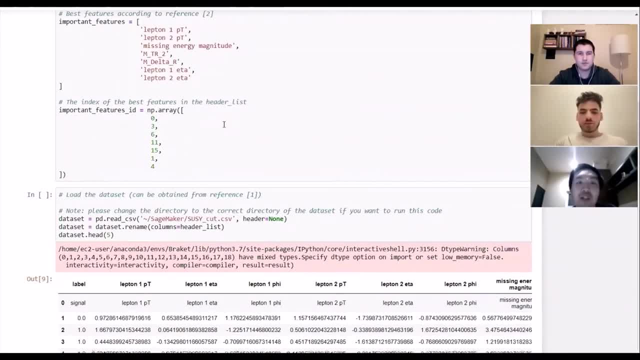 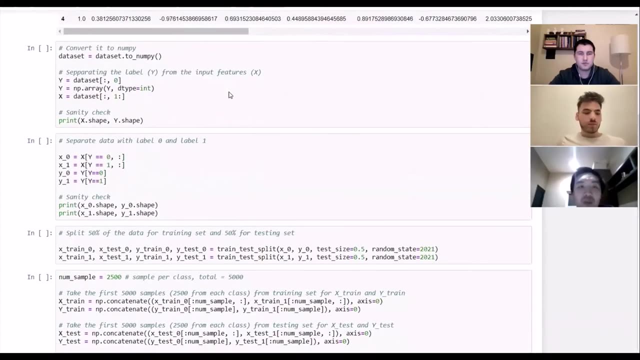 The top 6 of the features, based on the reference number 2, is Clapton 1. PT. Clapton 2- PT. missing energy magnitude, MTR2, Mdelta R and Clapton 1 eta. Those 6 features are the one that we use for this implementation. 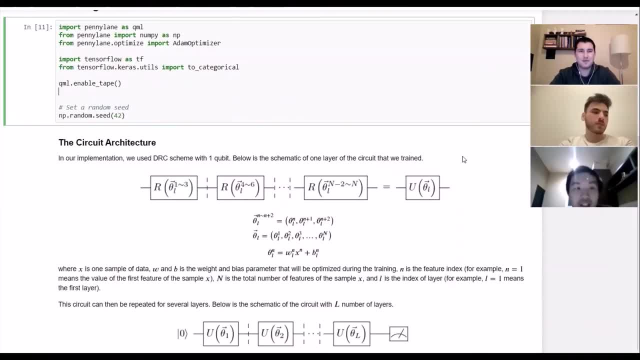 Next, this is the circuit schematic that we use for the DRC scheme. So we use the Penny Lane's rotation gates, Which receives the data set, Which receives up to 3 parameters, And because we use 6 features, So for every samples we need 2 sets of gates. 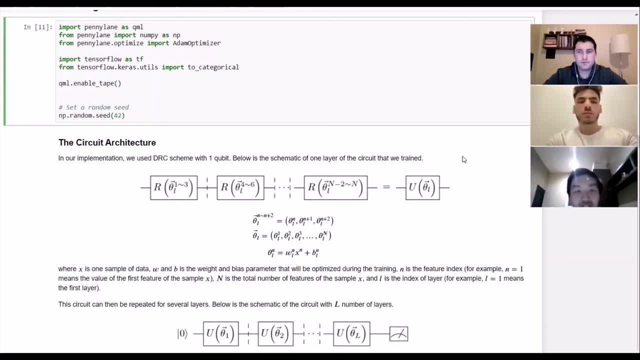 Because every gate will receive 3 features. And then this is the equation on how we embed the data into the parameters theta And then embed the theta into the gate. Okay, So we can see in this equation The W and B. here is the weight and bias parameters that will be optimized during the training. 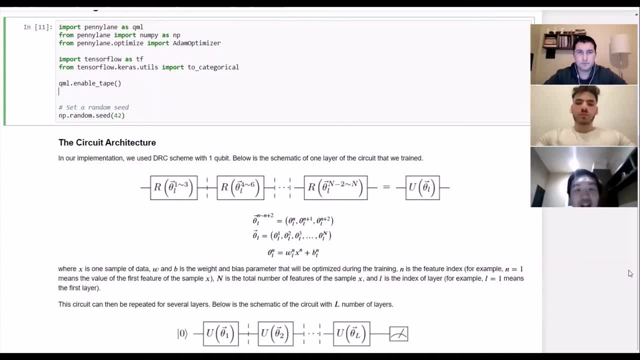 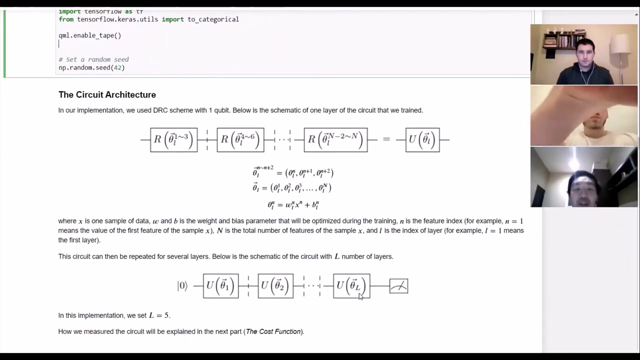 And the variable X here is the value of the data sample And the index M here shows the index for features And L here is the index for layer. So this block of circuit can be repeated for several times. In this schematic we showed that the block is repeated for L number of layers. 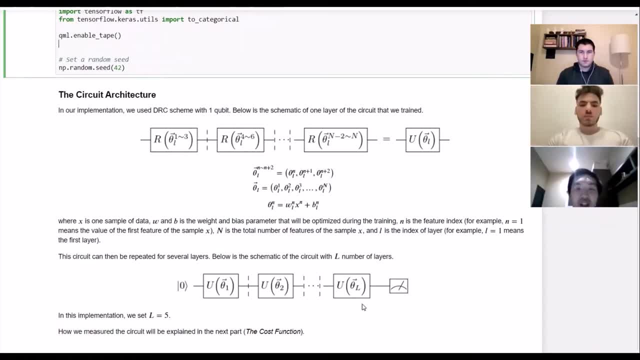 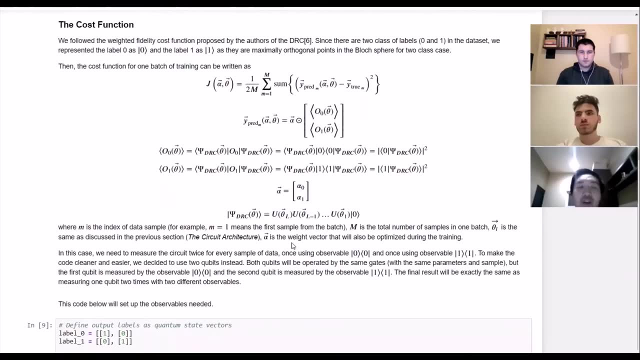 And in our implementation we set L equal to 5.. And then the cost function that we want to minimize. This is inspired from the original paper of DRC. So in the original paper the authors proposed the weighted fidelity cost function. 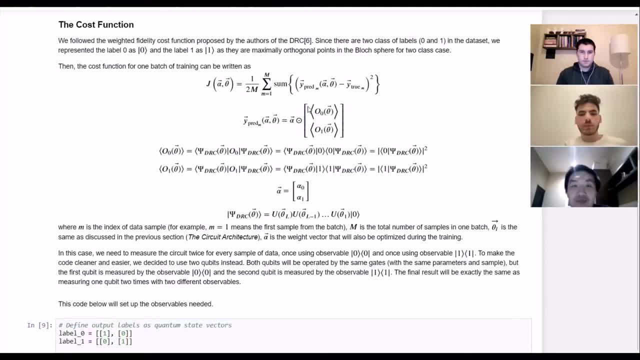 Which is this equation here? So we can see that the qubit we need, we only need one qubit, But we have to measure that. But we have to measure that qubit two times. The first one is using the 0, 0 observable. 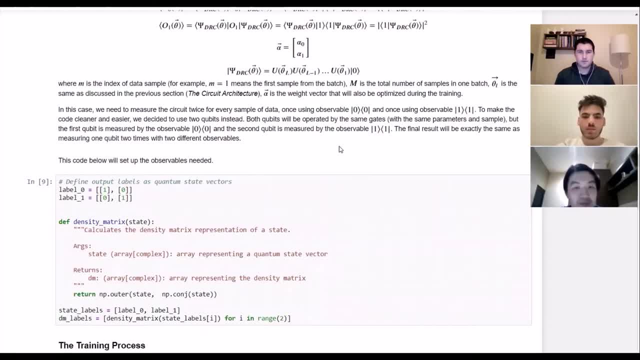 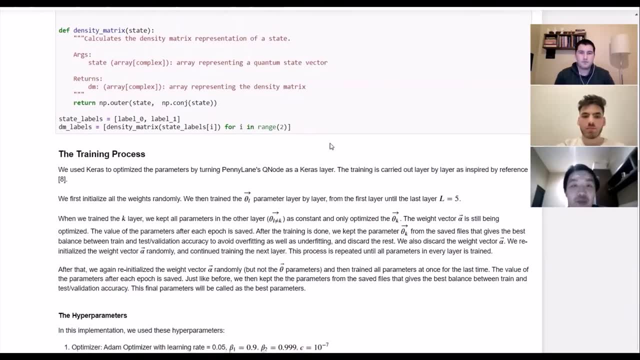 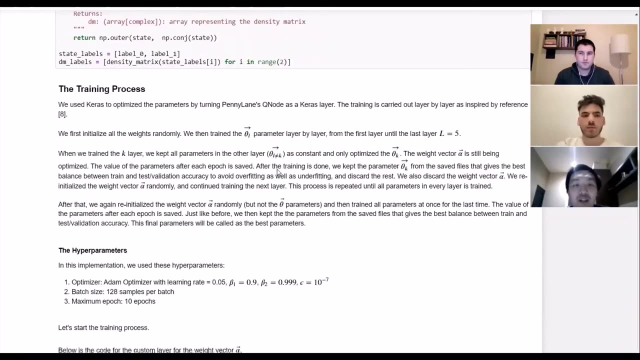 And the second one is using 1,, 1 observable. And then we train the circuit by using the modified version of layerwise learning, Where we train each parameters from each layer one by one. When we train the first layer, we make the parameters in the other layers. 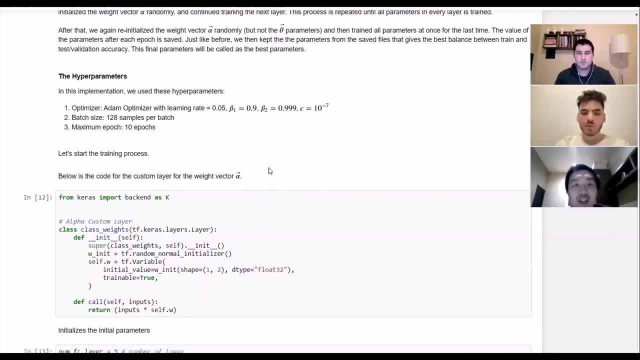 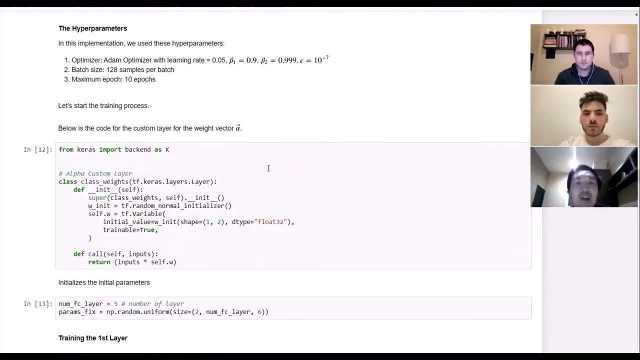 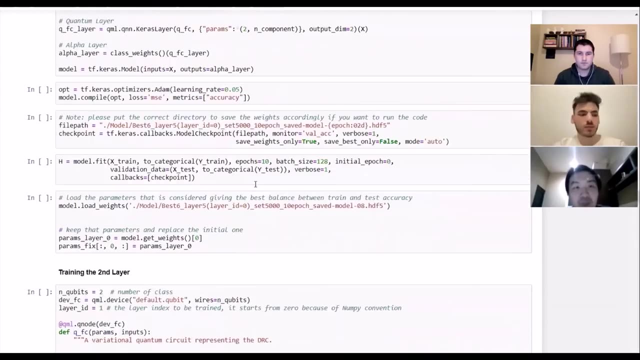 In the second and the third, etc. To be fixed. And then, after the first layer is finished, we train the second layer And we freeze the other parameters. We repeat the process until we train all the layers, And then the difference is we do the last training. 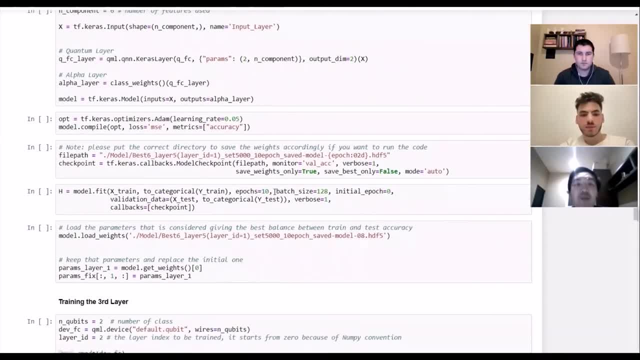 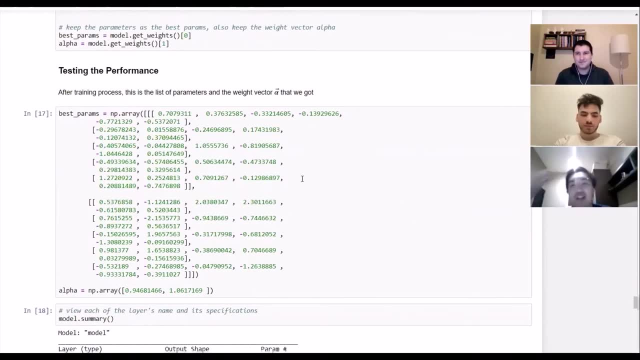 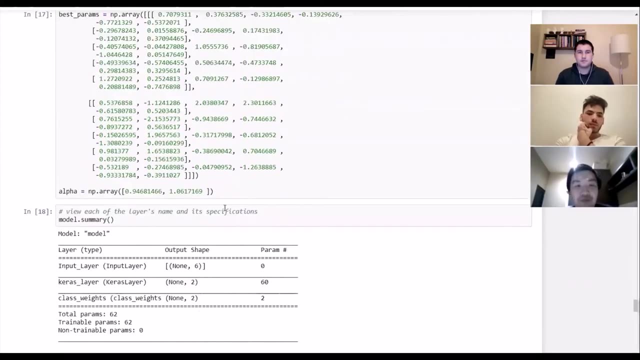 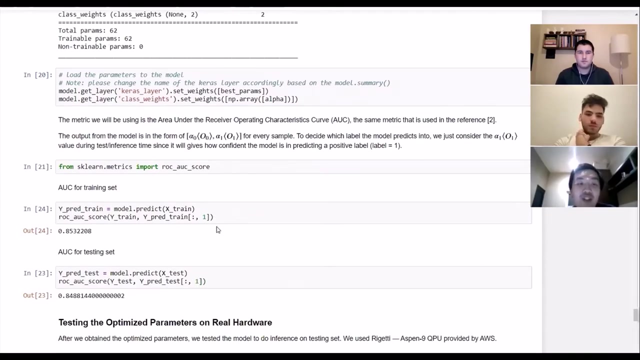 Which train all the parameters in all layers. After the training is finished, we test the performance of our model. This is the best parameters that we get from the training And from the testing results we get the AUC score on area under the rock curve. 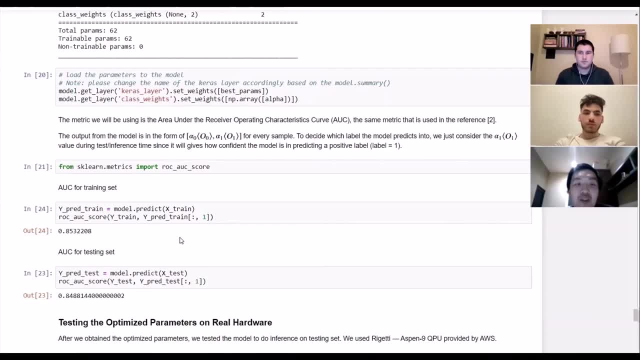 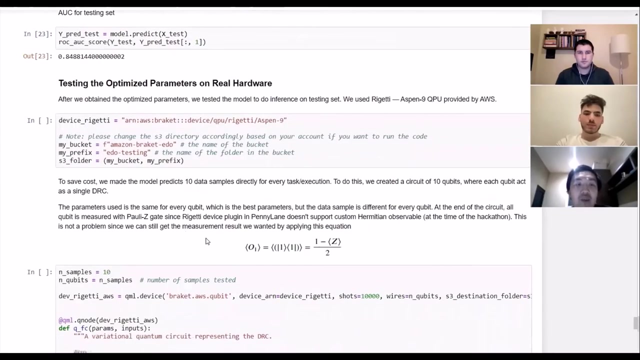 About 0.1.. 0.85 for the training set And 0.848 for the testing set. This number is a bit higher than if we compare the results that the reference paper number 2 gets. And then we also use that optimized parameter and try to do the testing on real hardware. 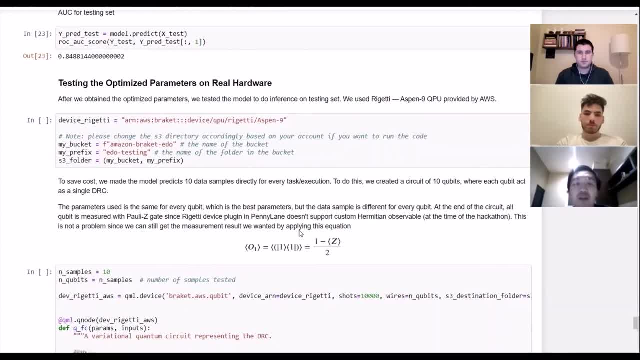 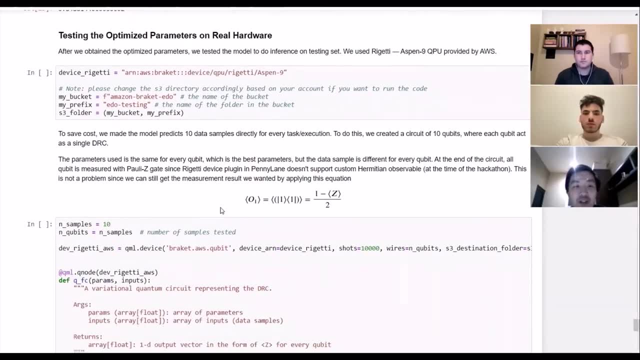 We use the Rigetti Aspen-9 QPU provided by AWS. Since the QPU device didn't support the 00 or 11 custom Hermitian gate, We use the Pauli-Z gate for the measurement And we can use this equation to get the same results as if we use the 11 gate. 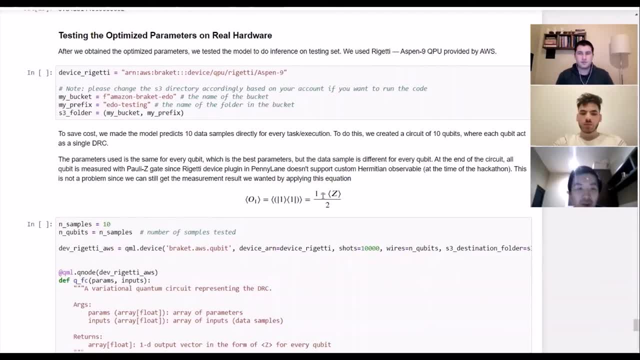 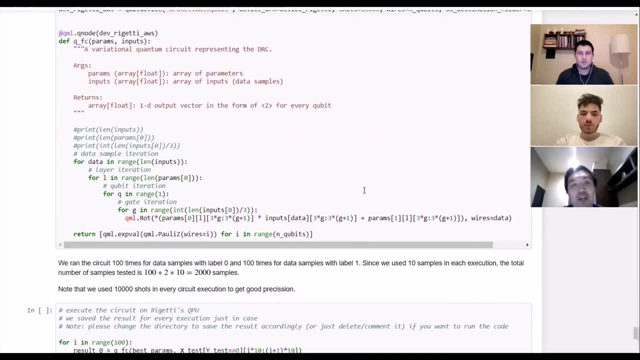 11 gate, 11 observable gate, And to make the cost become more efficient, we execute the circuit for 10 qubits. So even though we actually only need one qubit for every samples, we use 10 qubits. So for every pass we can get the results for 10 samples. 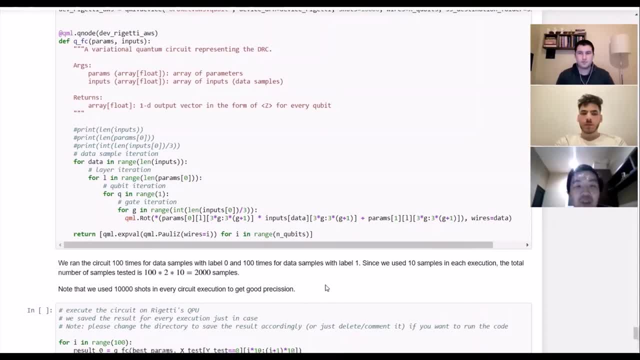 This way we can save the cost of the AWS device a lot. This way we can save the cost of the AWS device a lot. In total, we do 100 times of execution, both for the data samples with level 0 and with level 1.. 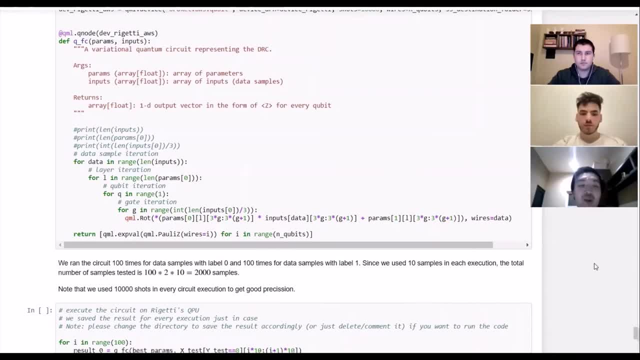 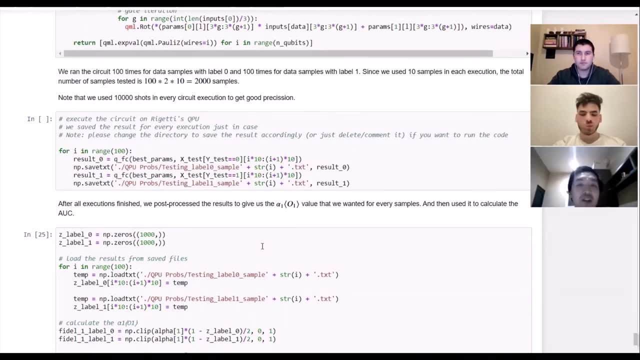 So in total we did testing with 2000 samples. So in total we did testing with 2000 samples And we used 10,000 shots in every circuit execution to get good precision. And we used 10,000 shots in every circuit execution to get good precision. 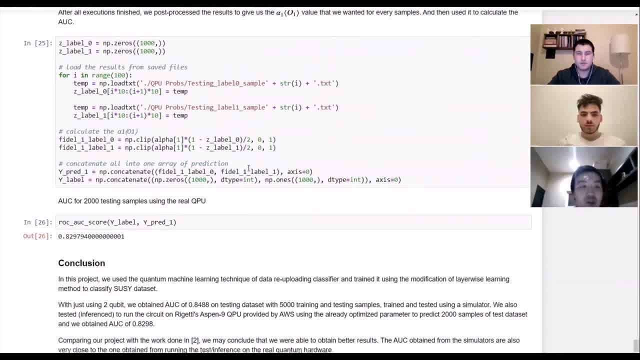 After everything is finished, we checked the AUC score and we got 0.8297.. Which is not so different with the one that we get from the simulators, And this result is also still better if we use it. And this result is also still better if we use it. 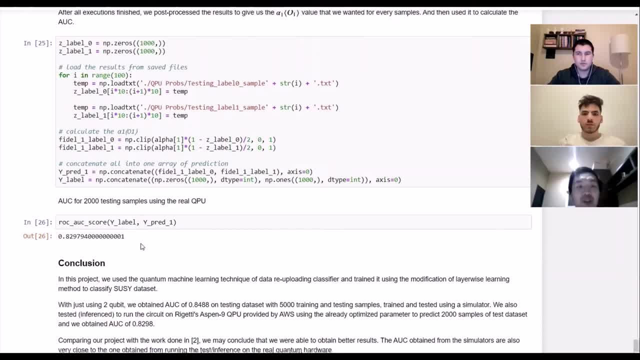 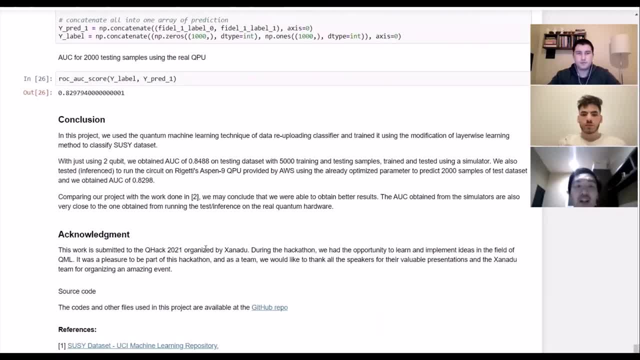 If we compare it to the one from the reference paper number 2 that they got with the Veo QPU device. In conclusion, in this project we managed to build an algorithm and to train the quantum circuits to classify the SUSI dataset. 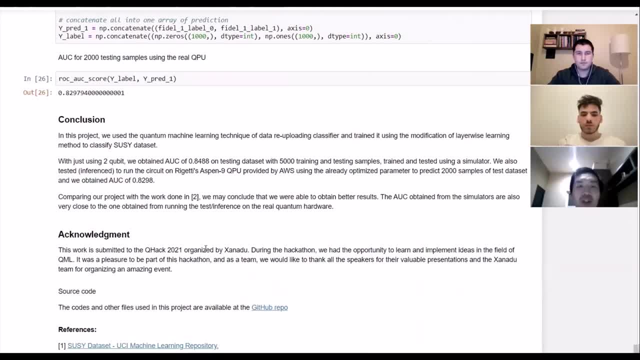 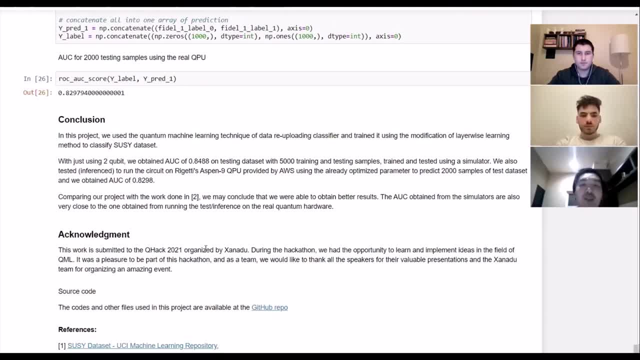 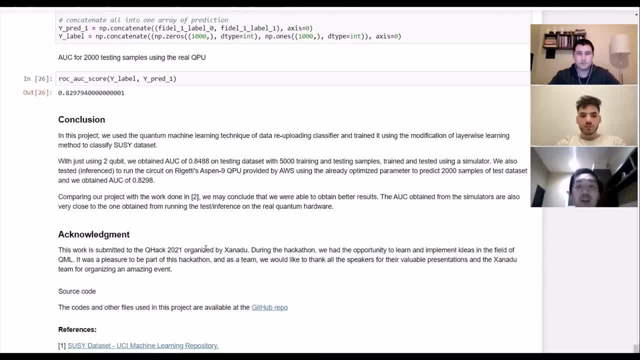 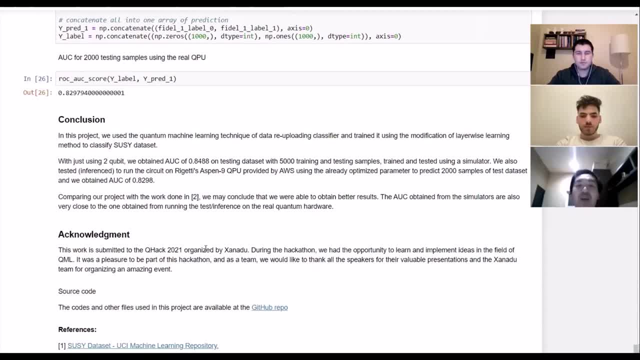 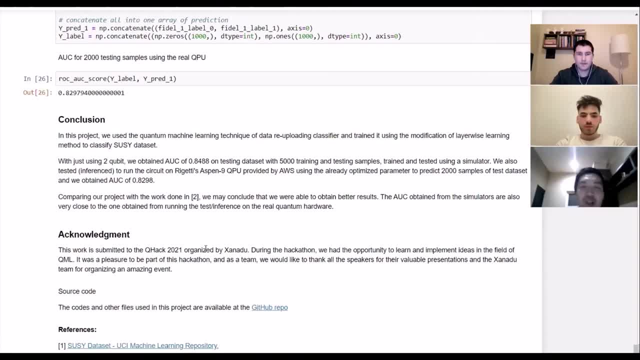 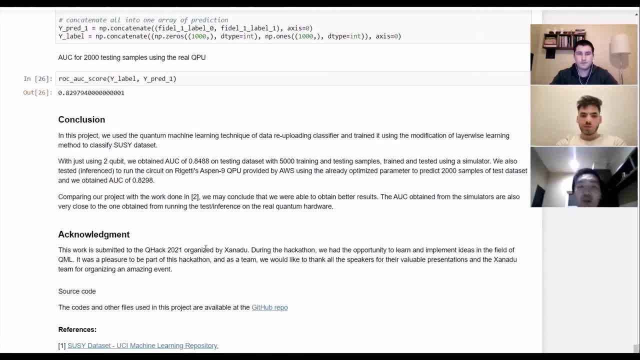 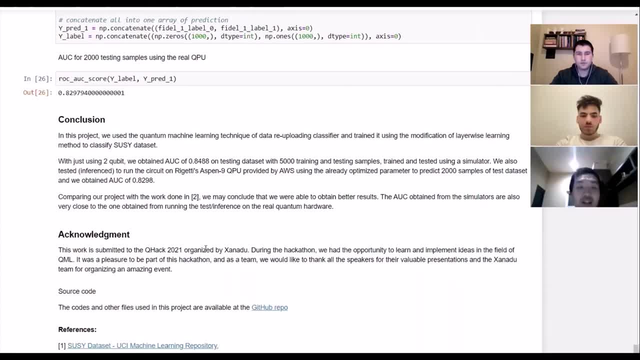 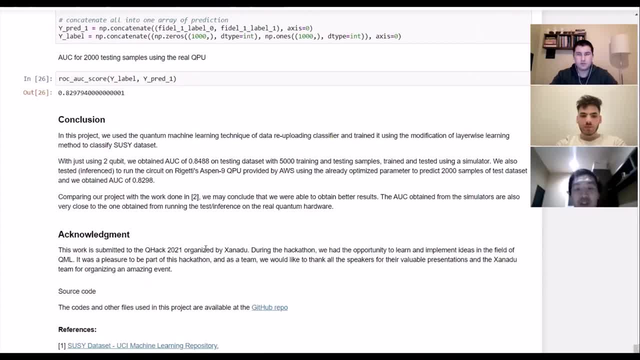 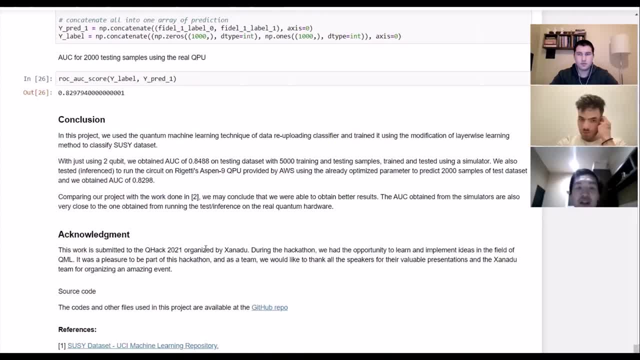 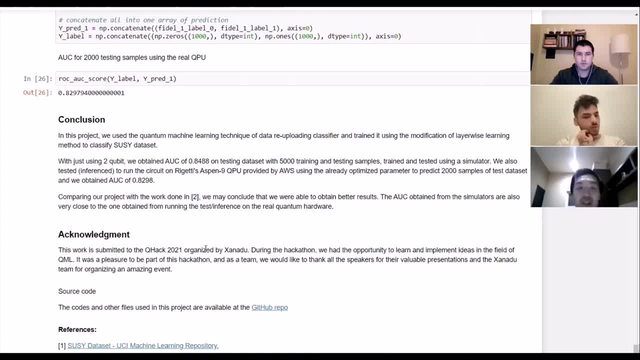 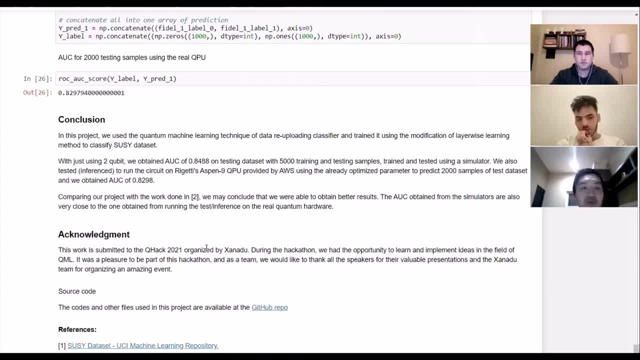 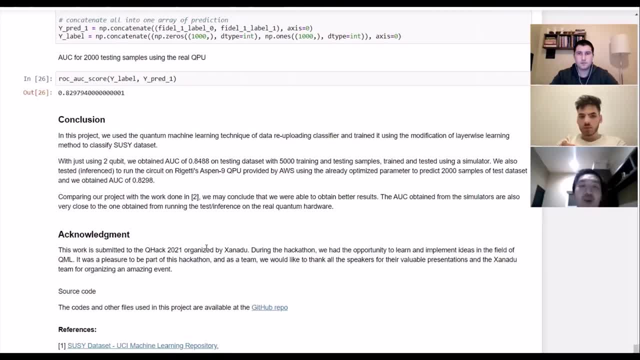 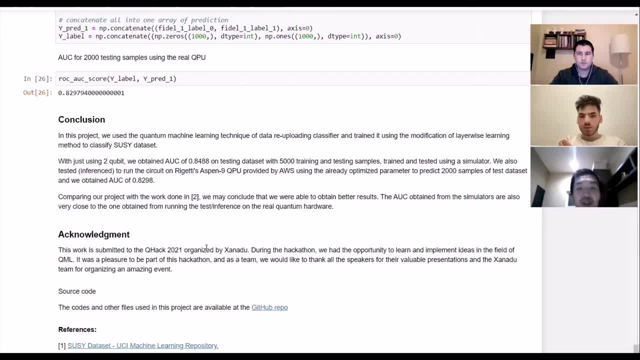 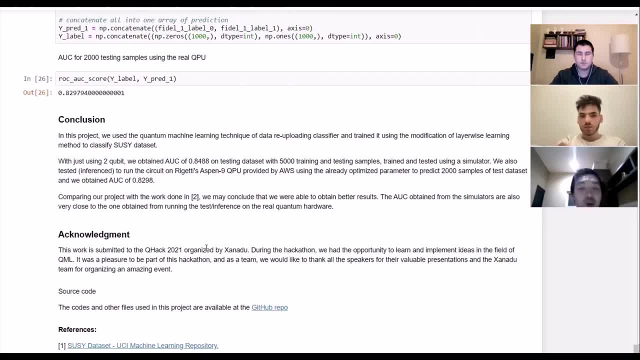 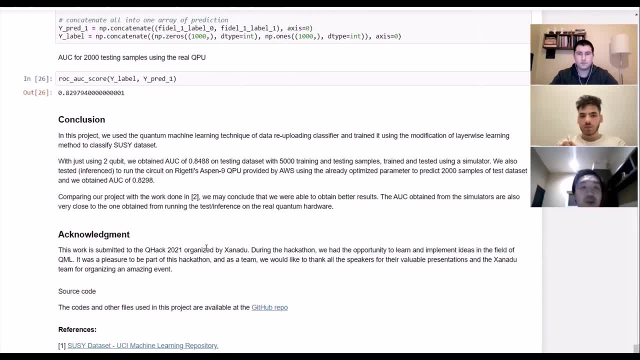 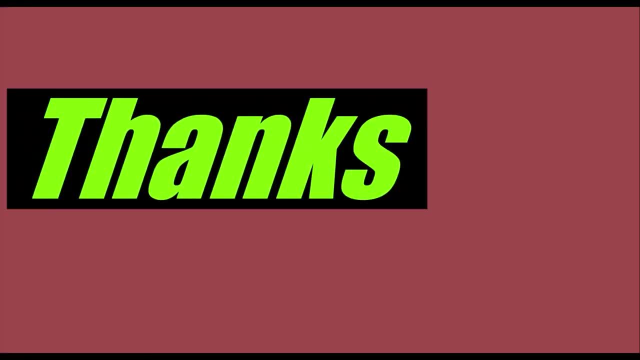 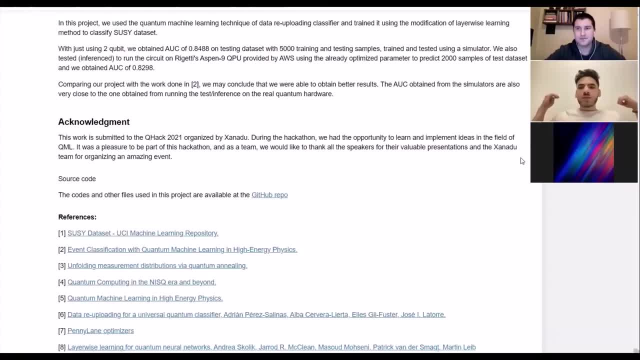 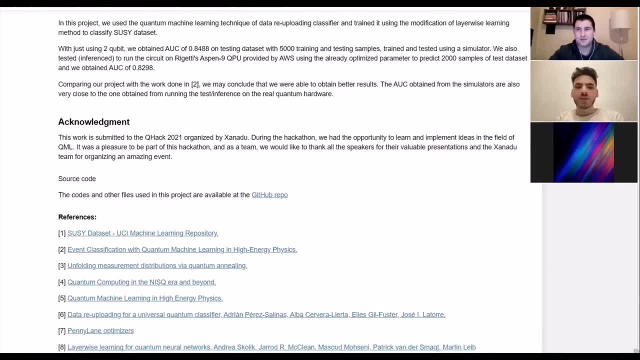 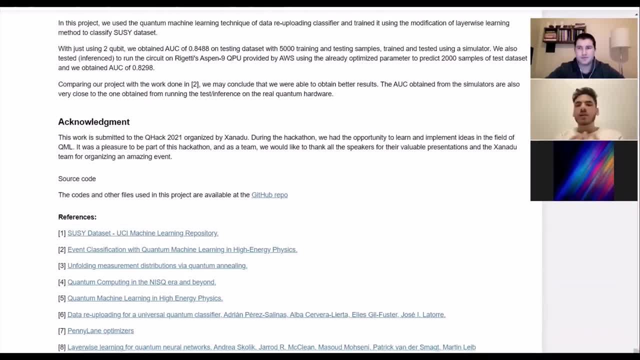 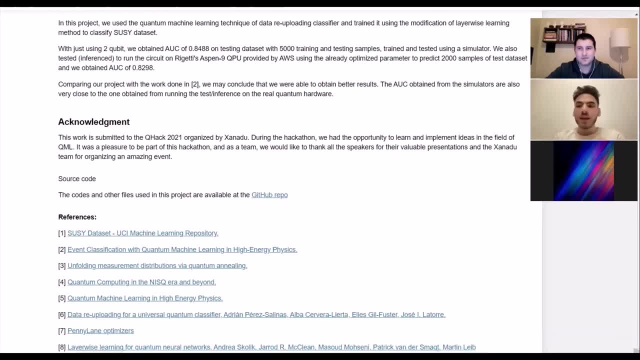 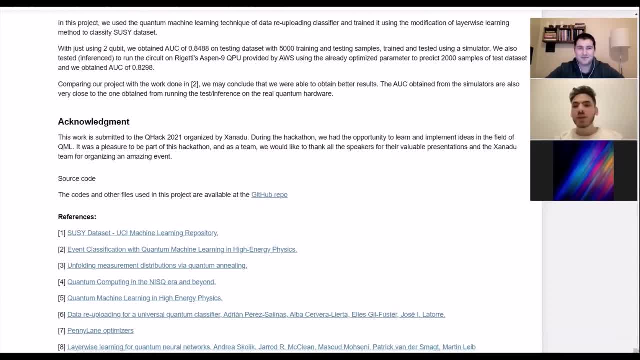 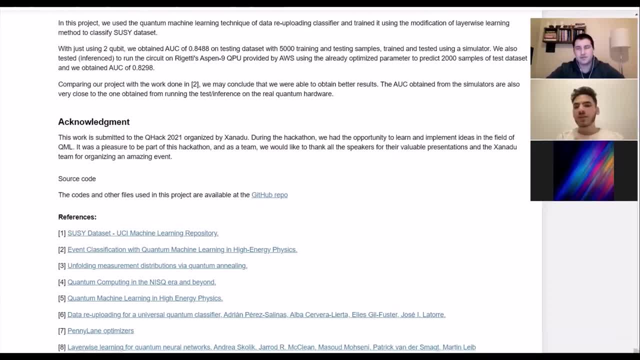 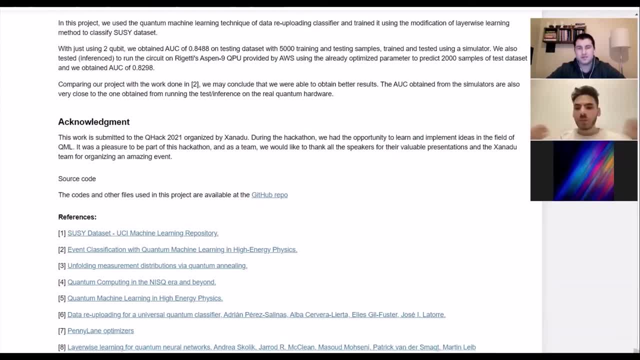 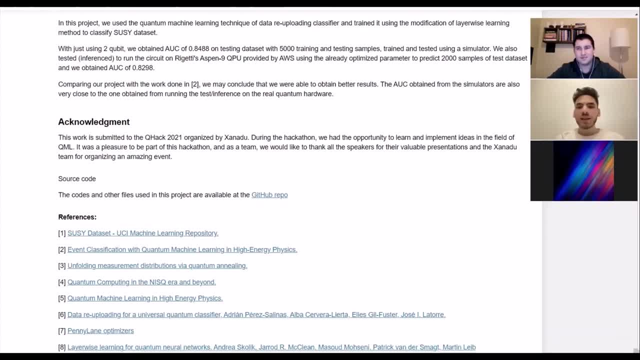 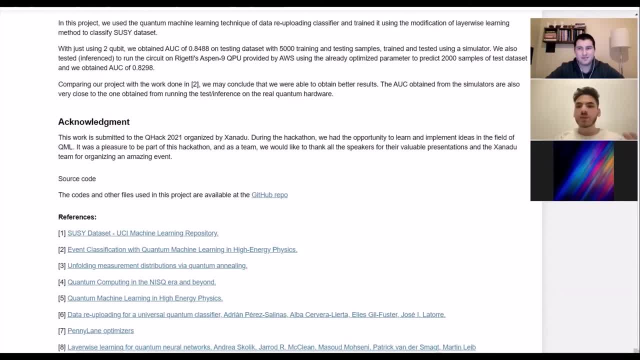 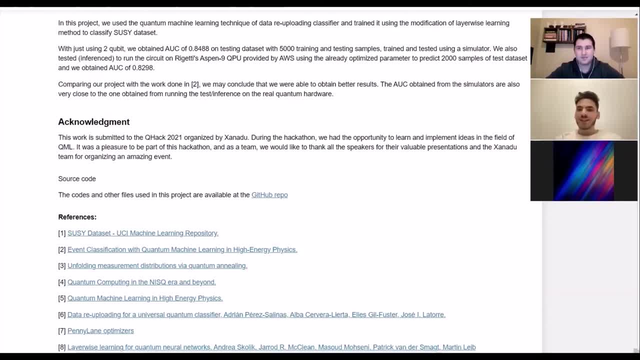 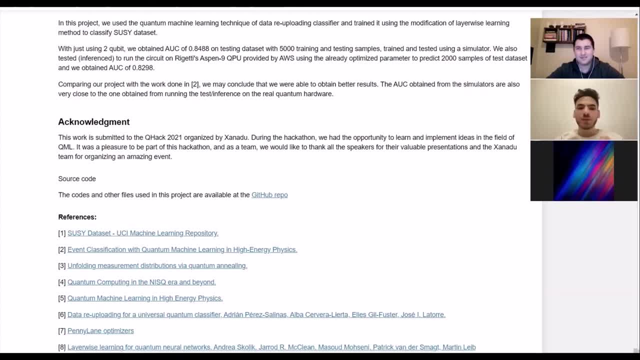 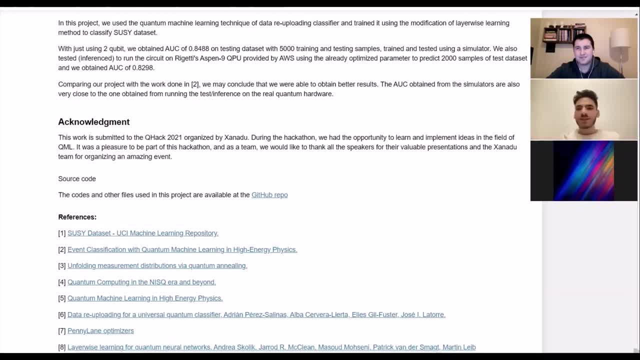 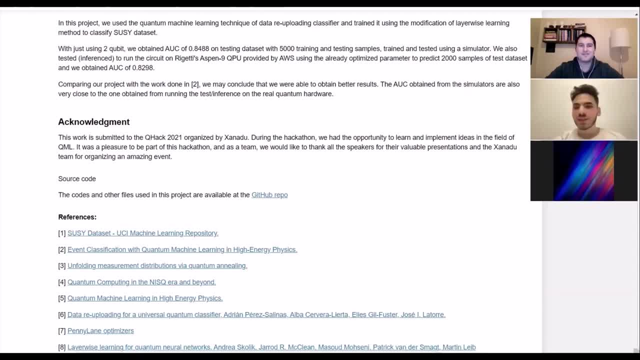 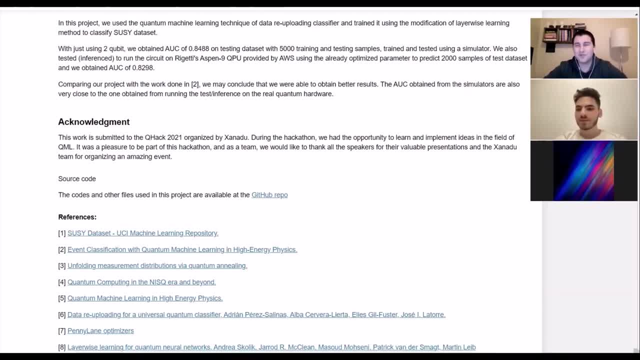 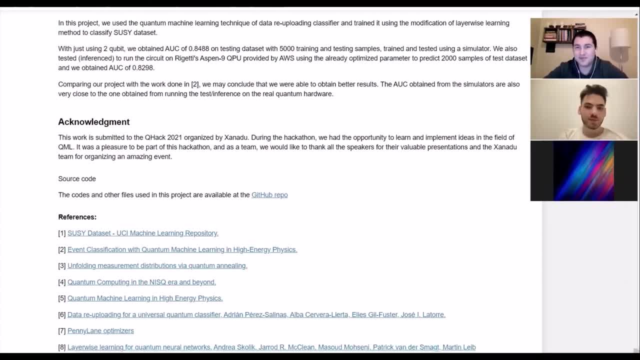 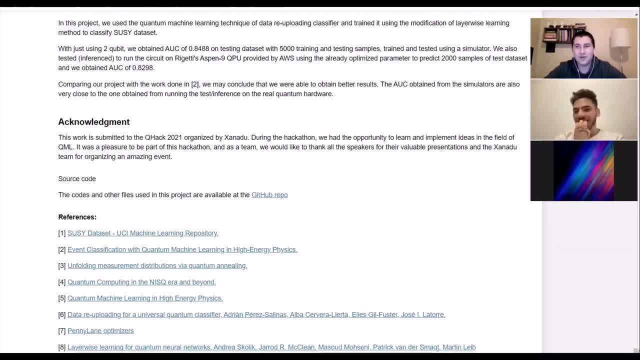 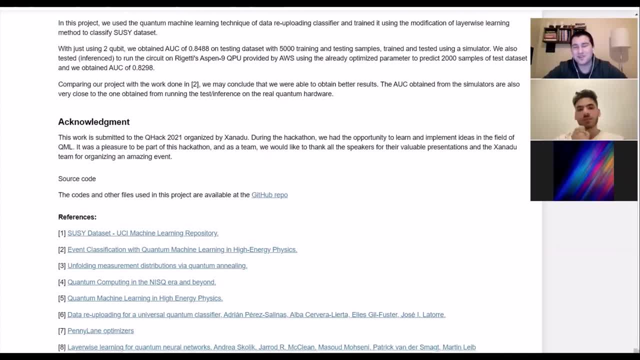 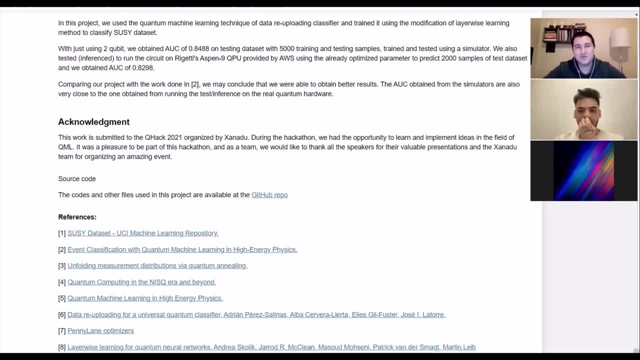 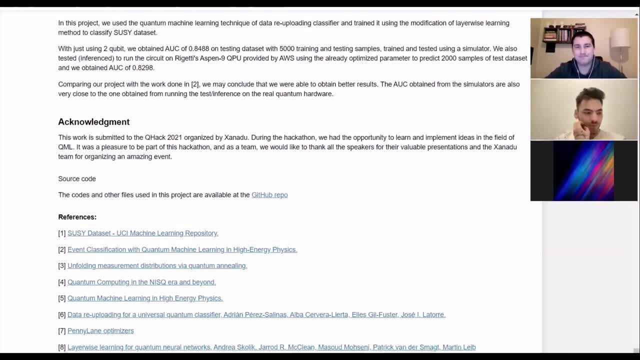 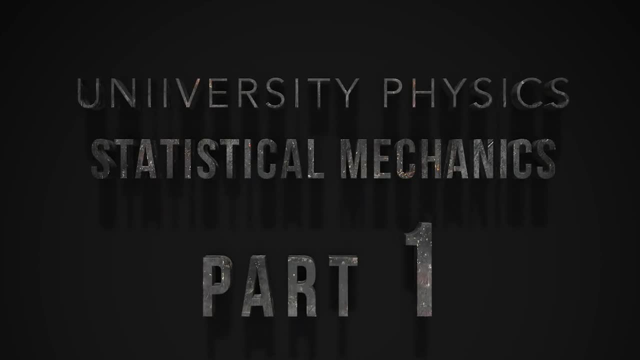 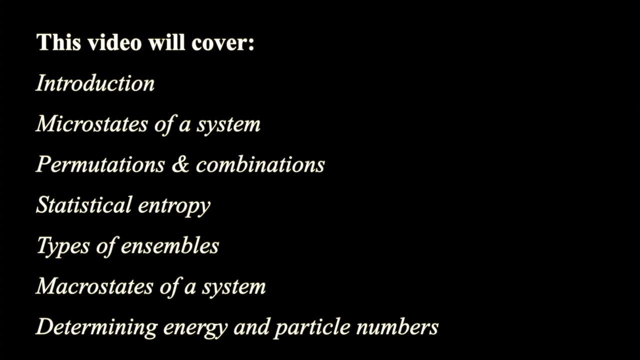 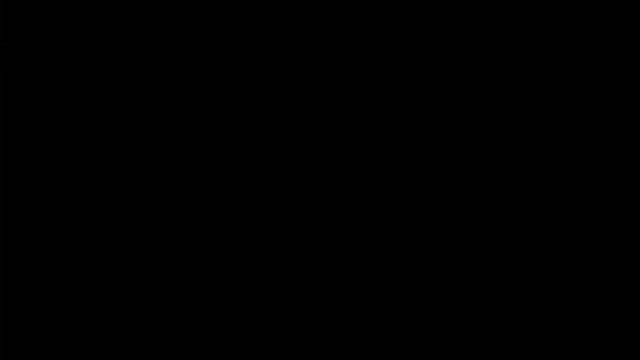 Hey guys, and welcome to another video in my series of university level physics videos, and in this video we are going to be kind of continuing our video series of thermodynamics. however, in order to get any further, we need to go on a bit of a slight detour, so we've kind of just we've, we've. 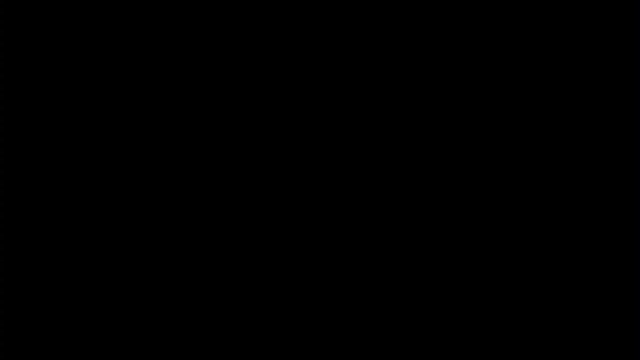 done the first, second and third laws of thermodynamics and that this kind of takes us up to about, you know, 1800s. so by this point we can kind of do things like steam engines and fridges and cool stuff like that, cool stuff like that. but it does go a bit deeper, thermodynamics, and in 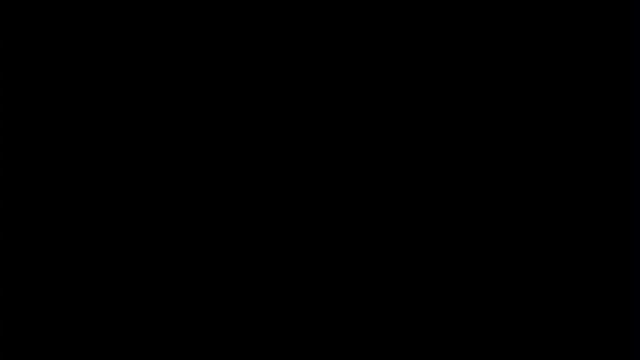 order to go any deeper, it's actually we actually have to go into the wonderful realm- or probably not so wonderful, if you're like me- of statistical mechanics. and when I first heard statistical mechanics I was like what the hell is this crap like? it's very abstract at first, and at first I really didn't understand it or like it very much, to be honest. 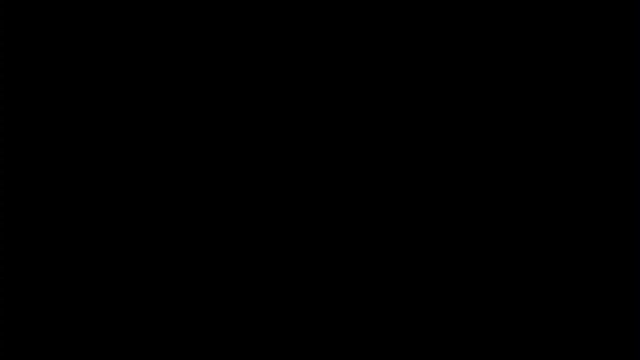 however, I do feel I'm at a point where I can probably explain it in a in a simple way. I know that it can probably be a little bit daunting at first when you start doing statistical physics, because often you've just finished doing thermodynamics and then you're all of a sudden